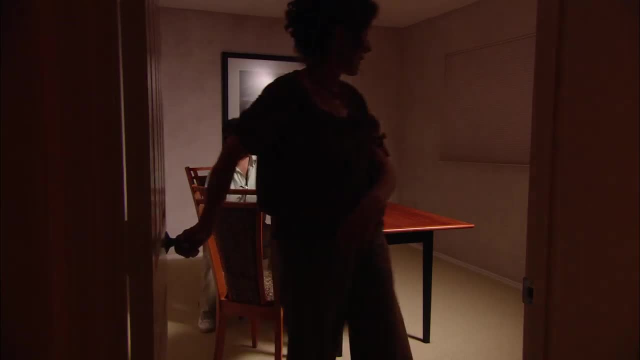 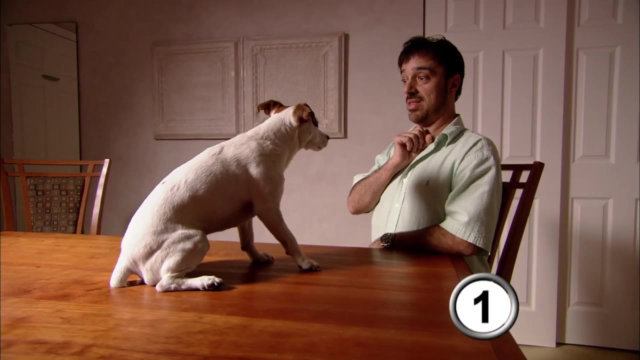 Good luck, Meg. Finally, DeFranco sets up the ultimate test and asks Jessie to leave the room. Maggie, Good girl. Six plus one. With Jessie out of the room, Maggie seems to be able to move on, But she becomes unable to get the right answers. 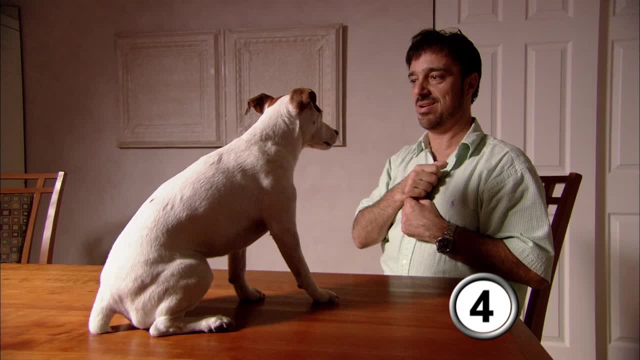 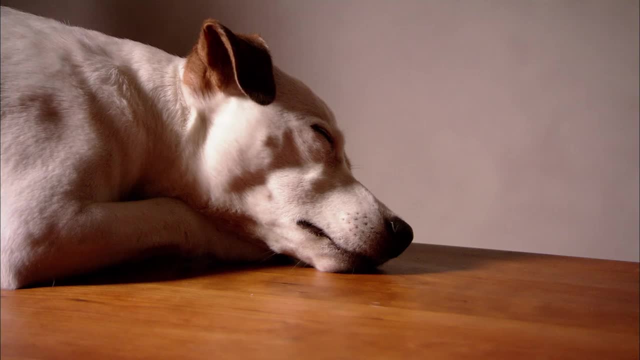 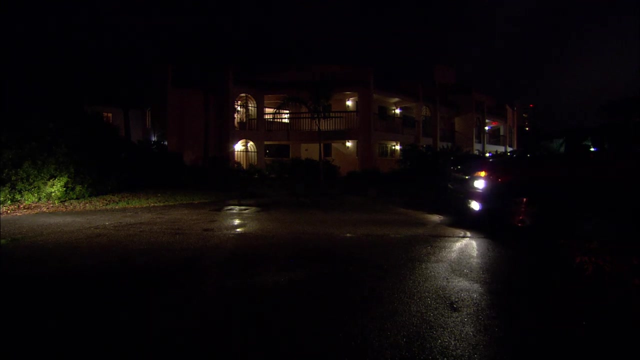 Maggie Six minus two. Okay, I'm not able to duplicate it. DeFranco is satisfied that he has proved his point. Maggie can only get the answers right when Jessie is in the room, So Maggie must be picking up invisible signals from her owner. 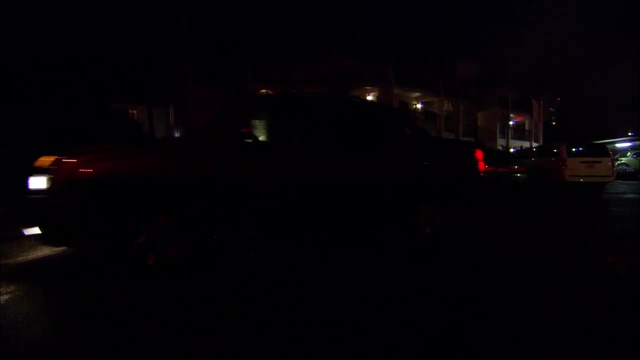 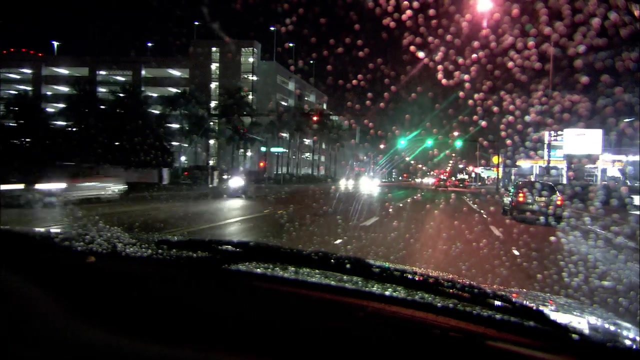 But what these signals are he can't explain. There is something that's going on in the room when Jessie is there that's not going on when she's not. So we can conclude from that that Maggie in some way is taking some cues. 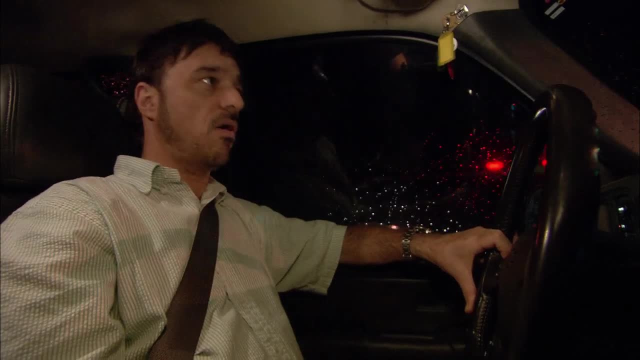 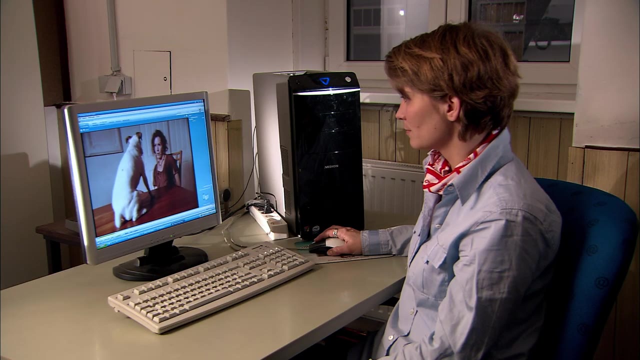 from something that Jessie is doing, whether or not she's aware of it. Over in Vienna, Frederica gets a chance to look at DeFranco's test And she's extremely impressed with Maggie's ability to focus on Jessie, So she's watching very closely what the owner is doing. 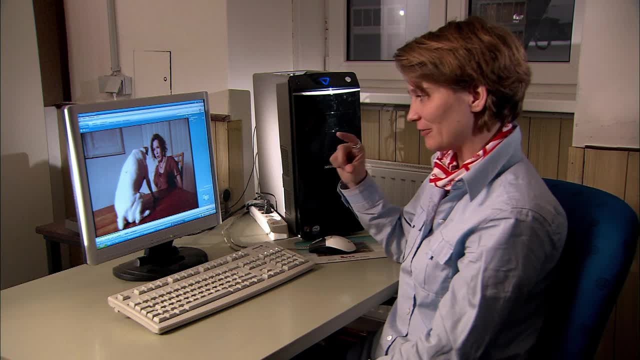 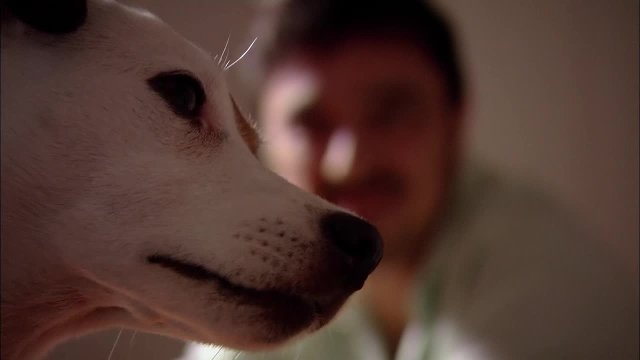 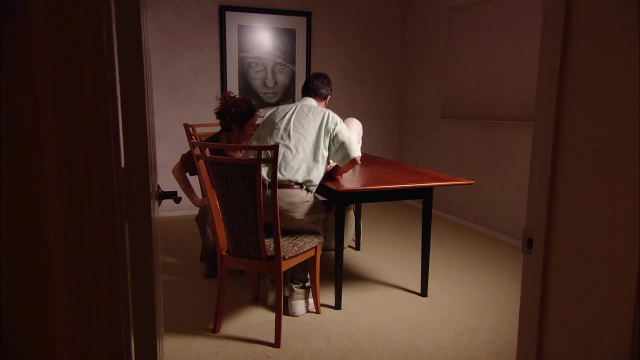 She's watching the face Very, very intensely. I've seen a dog being so concentrated on something, So she's looking for something there, But Frederica can't see any obvious cues or signals from Jessie. With Jessie out of the room, Maggie appears to reveal her technique. 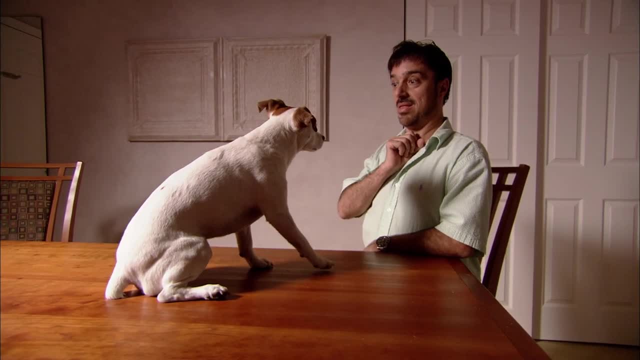 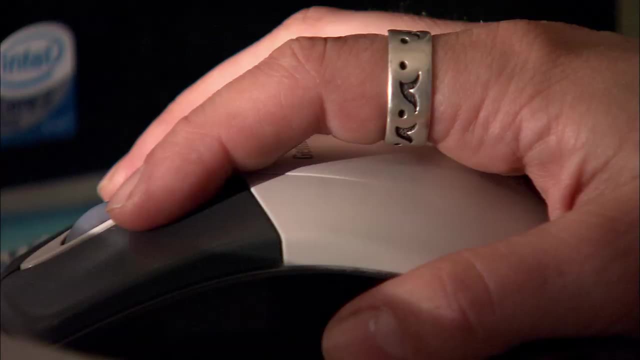 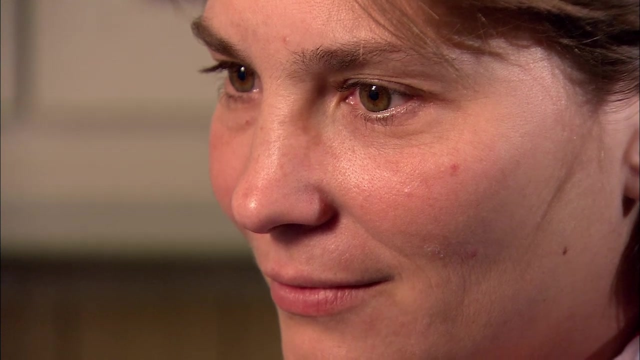 She is clearly influenced by DeFranco's nodding head Here. it was very clear that he's nodding the head. Well, counting My cues don't have to be deliberate. They can be unconscious If you're focusing on something and you're expecting something. 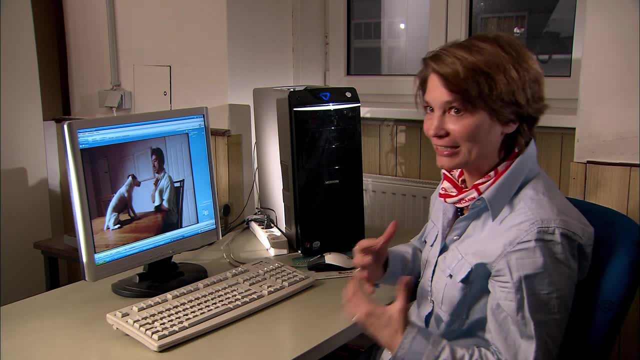 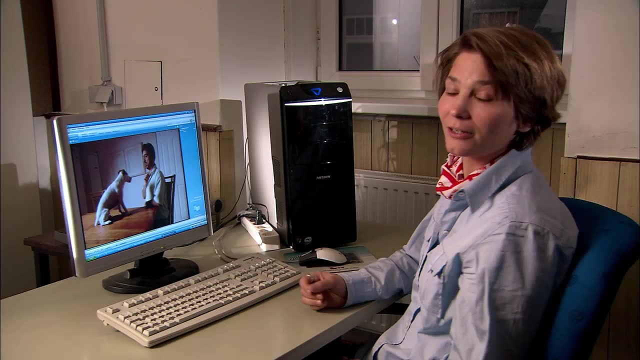 you know the answer. it's very easy to get into that movement or giving some other cues within your body that you really don't have any control about. He probably didn't do it consciously, He just did it unconsciously, But there were cues there, lots of them. 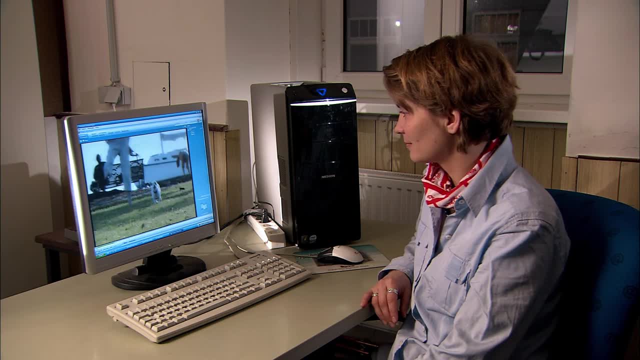 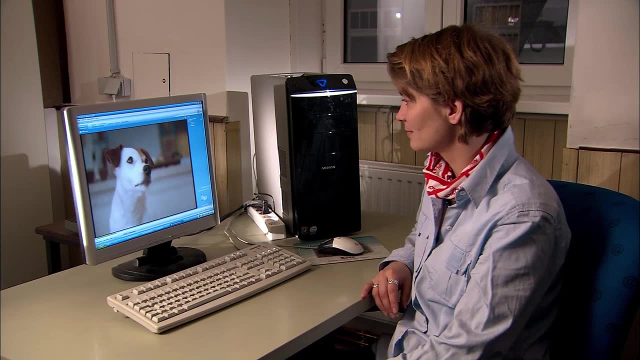 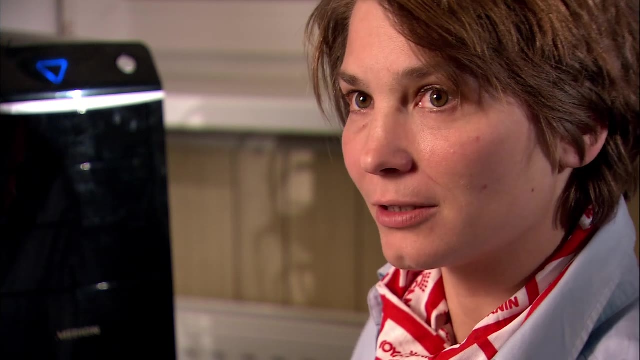 So Frederica still believes that Maggie is an extraordinary animal, Not because she can do maths, but because she can pick up on the tiniest clues in her owner's face and guess what she's thinking. I've never seen such a high level of attention to these features.